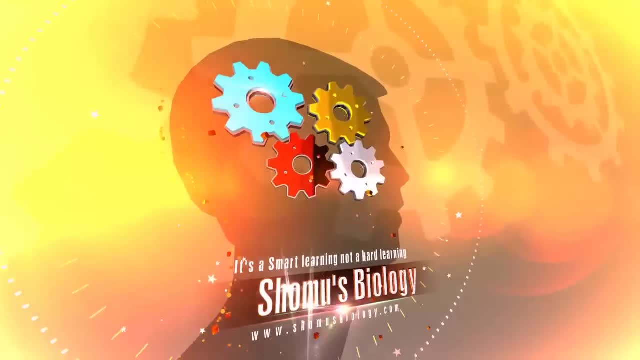 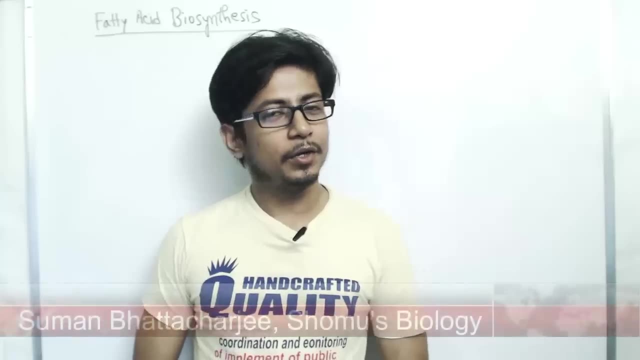 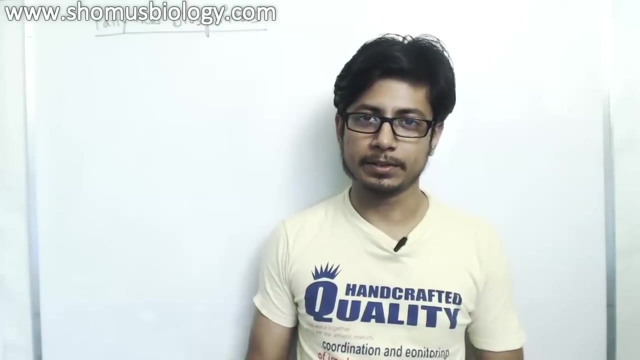 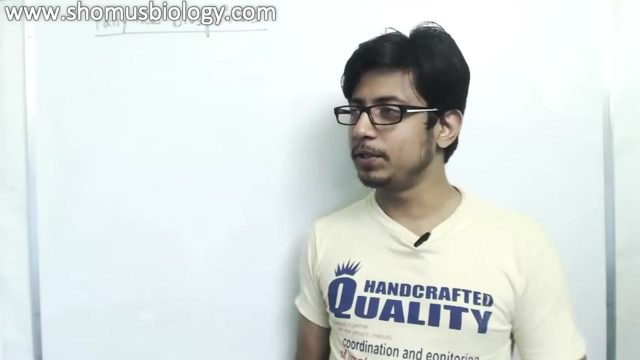 Hello friends, welcome to another video tutorial from show most biology and the series of videos we are talking about metabolism videos, and mostly in the last couple of videos we talked about carbohydrate metabolism, But from this video we are going to talk about fatty acid metabolism, especially three part of the fatty acid metabolism. 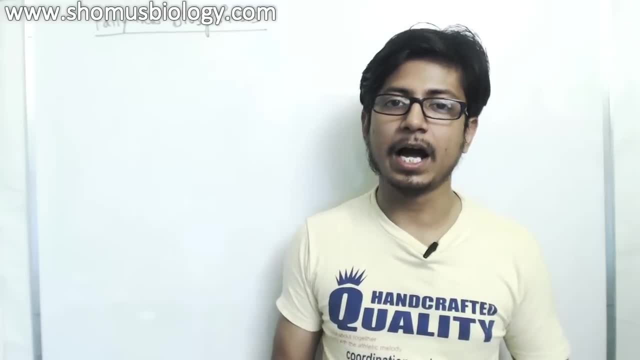 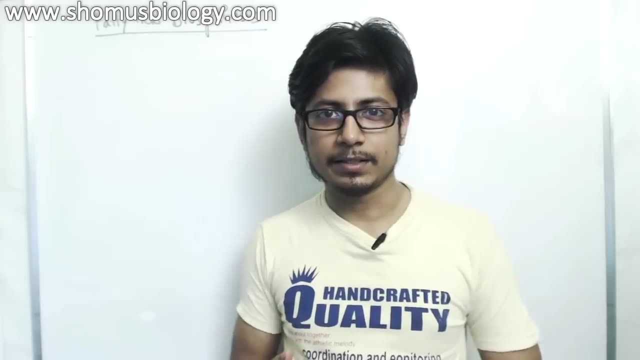 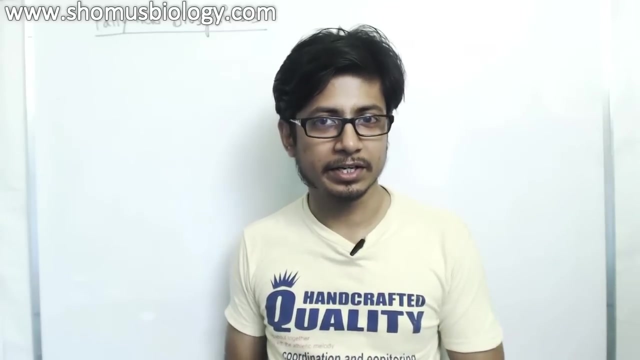 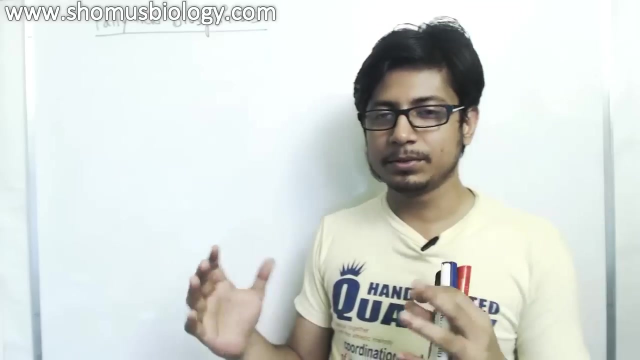 First is the overview of how fatty acid after digestion is utilized in your body with the help of different receptors. Second part is the fatty acid biosynthesis and the third, fatty acid beta oxidation. that is, the fatty acid degradation. Now the second part of fatty acid biosynthesis is the topic of this video. The term you see: the production of fatty acids in our body. Now we all know the important. 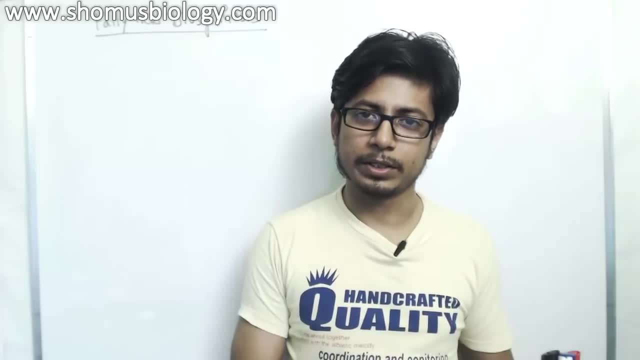 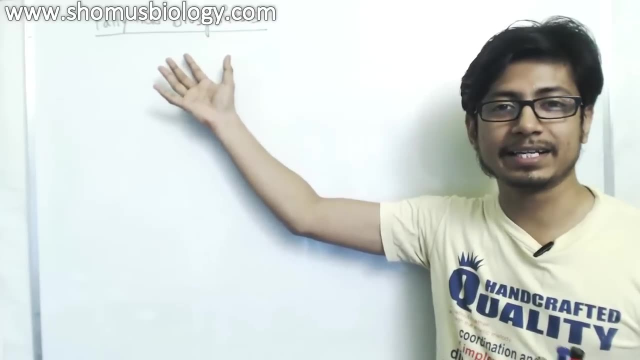 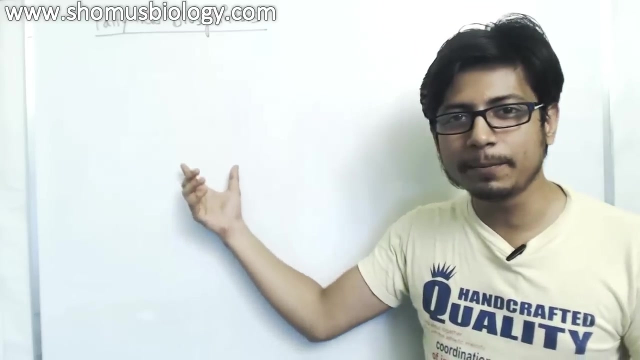 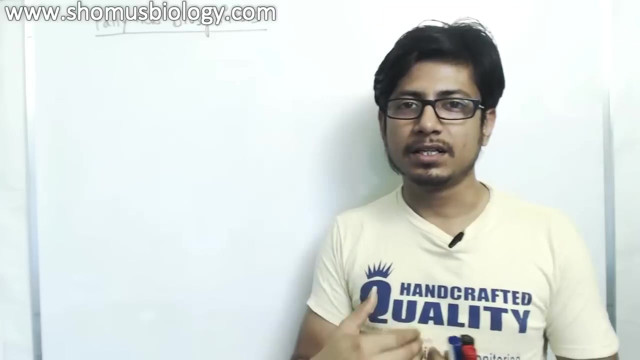 of fatty acids and all the other fat molecules in our body. They are really highly energy conserved molecules. So for making such a high energy producing molecule will also require a lot of energy from outside. So in this anabolic pathway of producing fatty acids we need several ATP molecules to involve with and also we need a starter molecule that will start the process. So in this case the starter molecules that that begins the process of fatty acid biosynthesis are acetyl Co A And NADPH. these are the two molecules that we need to start the process of fatty acid biosynthesis, And I told you that this NADPH- This is a product of pentose. 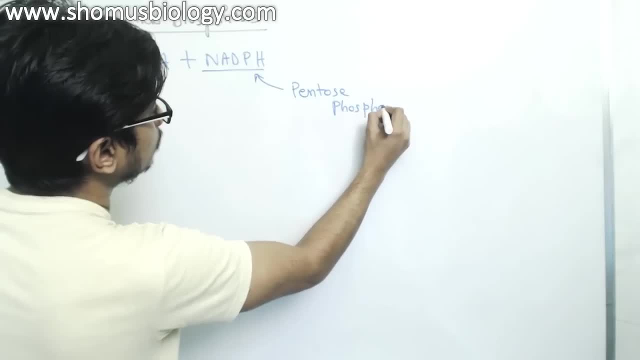 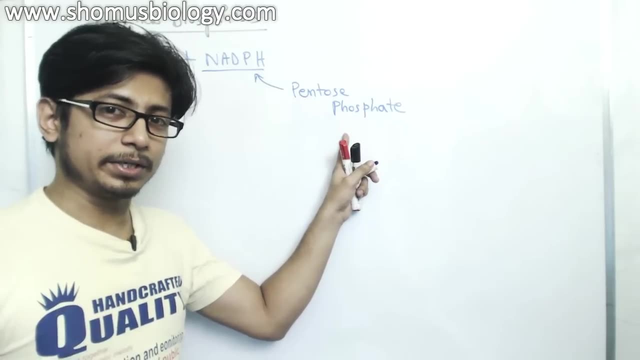 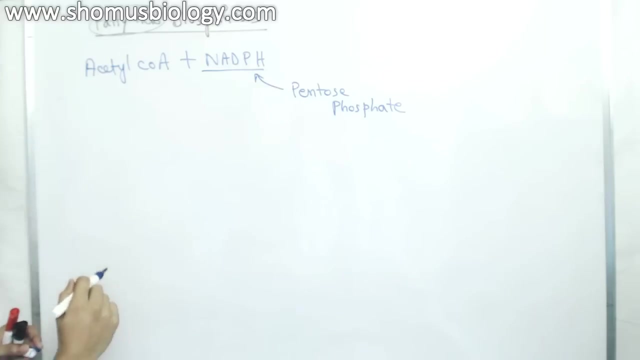 phosphate pathway. So if you check your concept earlier, Phosphate pathway is really important pathway because without it we cannot produce NADPH and without NADPH, fatty acids cannot be produced. That's why it's very important to have NADPH concentration in our cell. Now there are 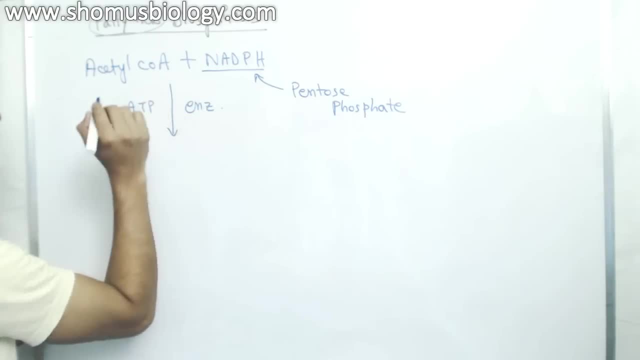 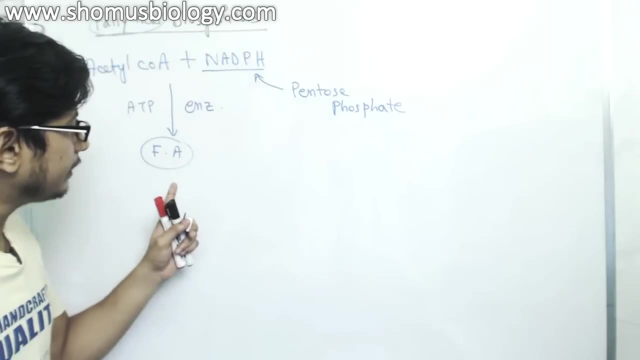 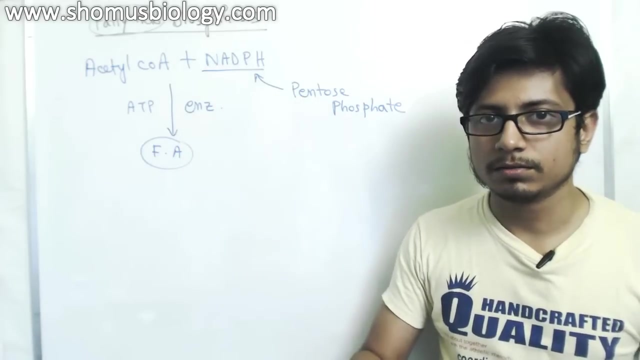 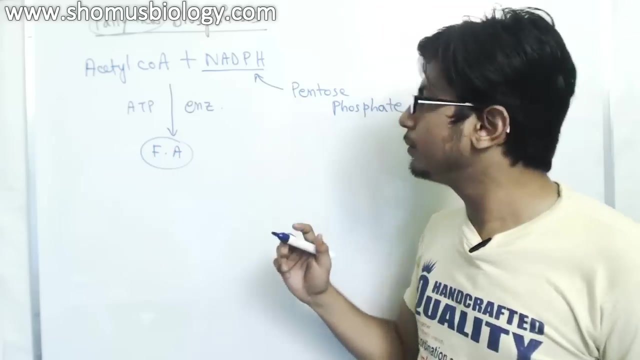 several enzymes and ATP molecules required to produce fatty acids. This is the simplest schematic that someone can give you The idea here. in this case of fatty acid production, If you think, the process works in a cytosol of the cell, So in the cell, cytosol acetyl CoA is required, so as NADPH, We know the pentose. 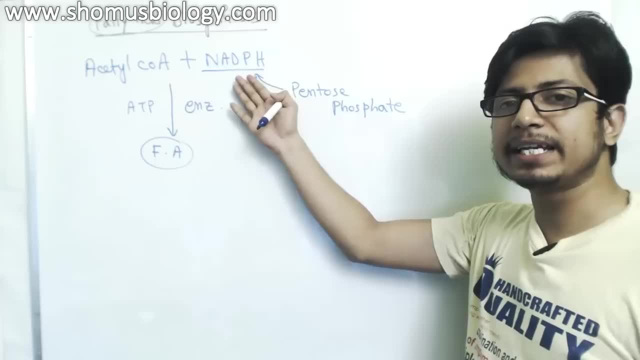 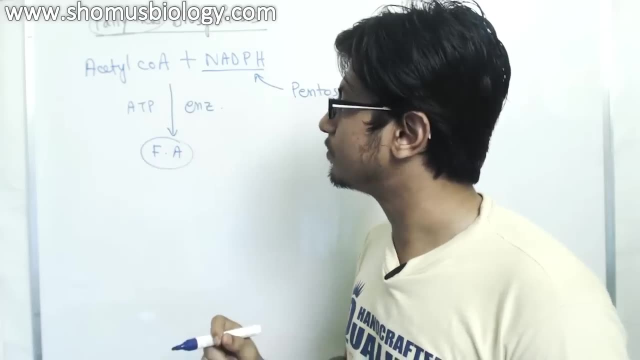 phosphate pathway occurs inside the cytosol, so NADPH can easily be produced there and can be utilized. but there is a problem with acetyl CoA to be brought in the cytosol, because acetyl CoA is not present in the cytosol normally. 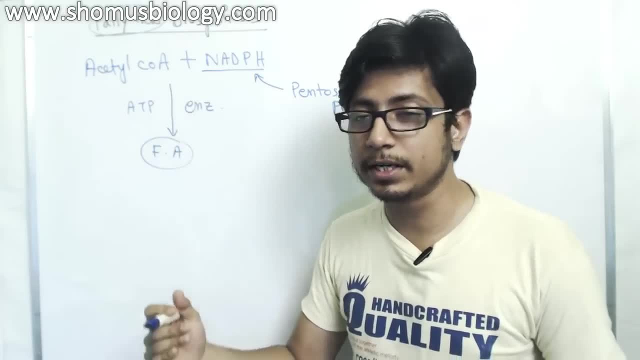 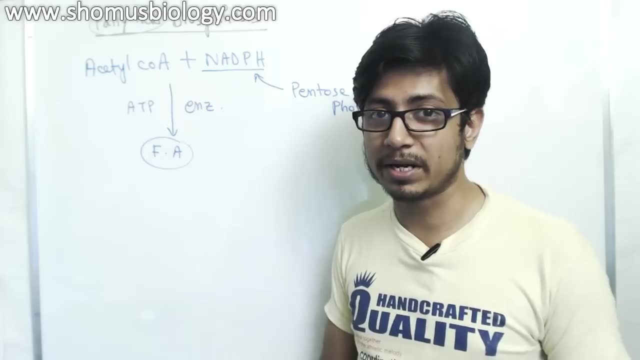 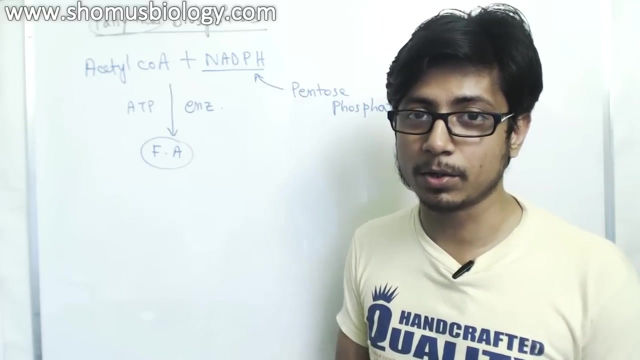 Acetyl CoA is produced, used from private, is converted to acetyl quay to private dehydrogenous complex. but that thing is done in the mitochondria and the matrix of mitochondria and we also know that acetyl quay cannot be transported across the membrane of mitochondria that creates the 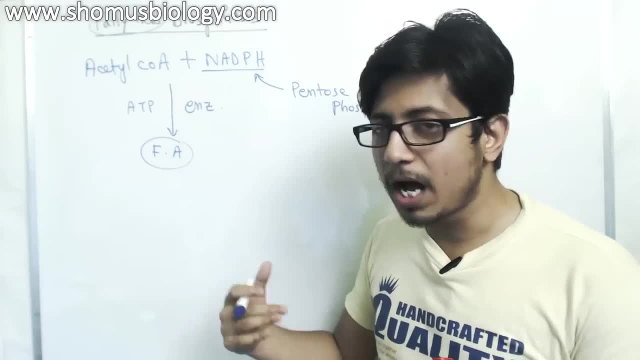 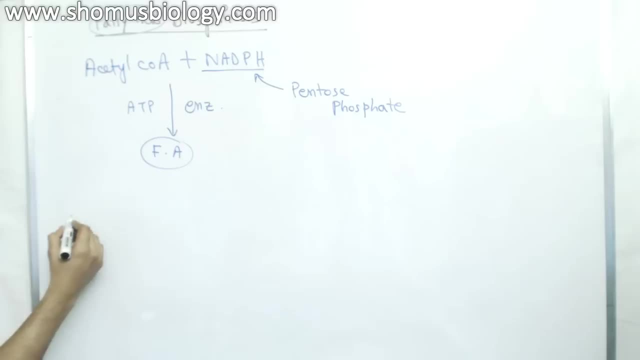 first problem of fatty acid biosynthesis, Now how we get acetyl quay in the site to solve from the mitochondrial matrix. and to know, that is, simply know, if I, if I draw the mitochondrial structure. schematic drawing of mitochondria This is, let say, let say this is the membrane of mitochondria, somewhat looks like, and then 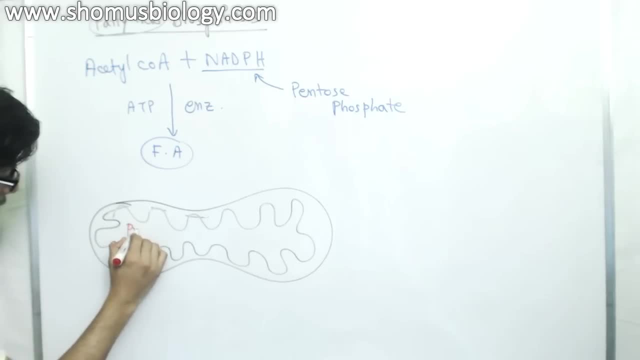 what happens here inside the mitochondria We we know we have the private, and private is converted to acetyl quay. Now there is no membrane channel through which the city can come out to the site to solve, But we know that inside the matrix of mitochondria 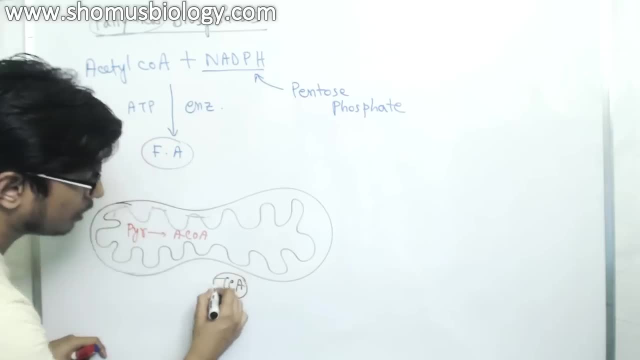 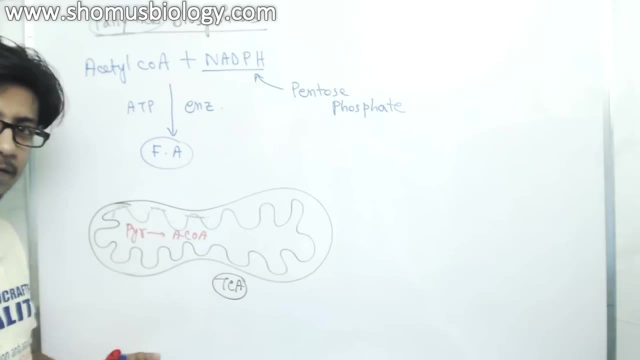 TCA cycle also carried out or Krebs cycle also carried out, and we know there are different Krebs cycle intermediates which can have the similar or which can produce acetyl CoA outside in the cytosol. so one such molecule that is there in TCA cycle is here citrate. so they 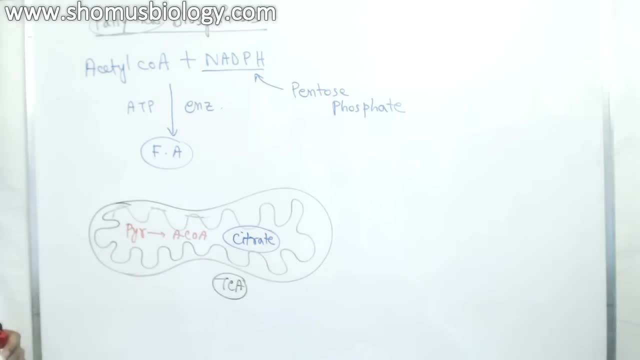 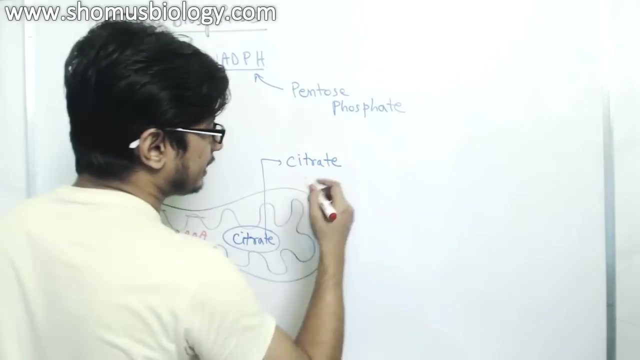 produce citrate inside the mitochondrial matrix. once they produce citrate, the citrate is released out. it can be easily released into the cytosol from mitochondria. so once citrate is out into the cytosol, citrate can be degraded. it can be broken down into two different part: one 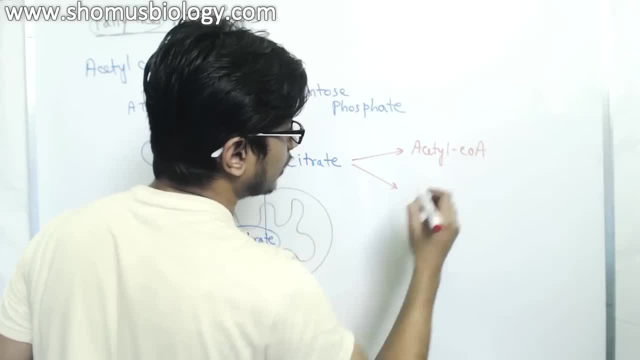 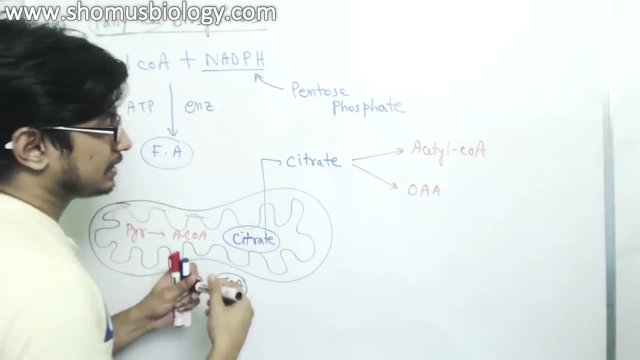 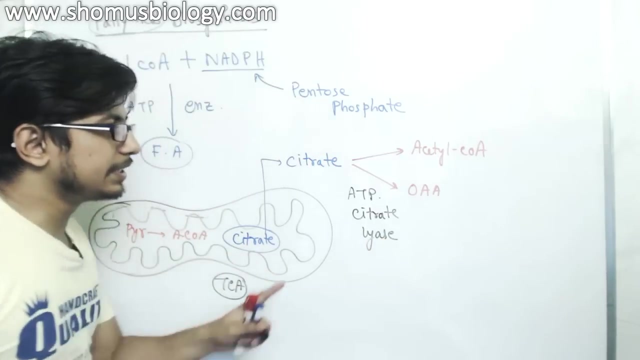 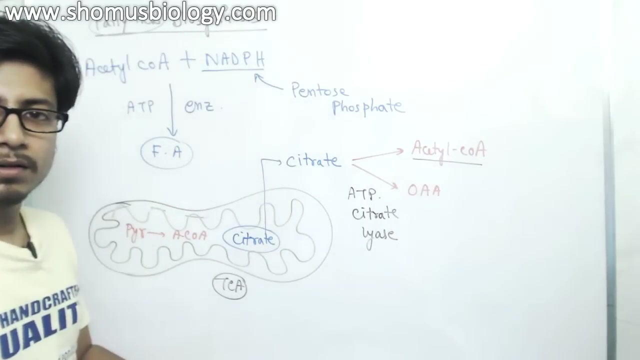 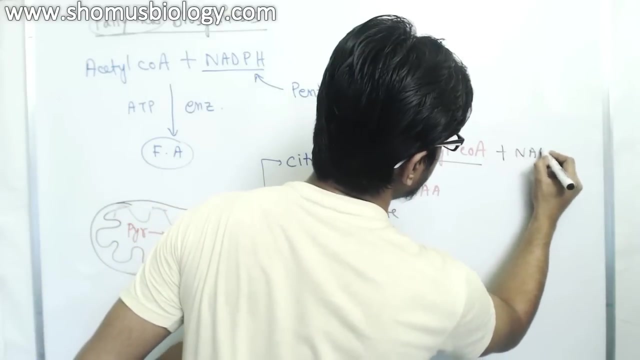 is acetyl CoA. another one is oxaloacetate. with the help of the enzyme known as ATP citrate liase, this enzyme breaks down citrate into acetyl CoA and oxaloacetate. now acetyl CoA can be taken for the synthesis of fatty acid with the help of NADPH, so along with NADPH, can form fatty acid. 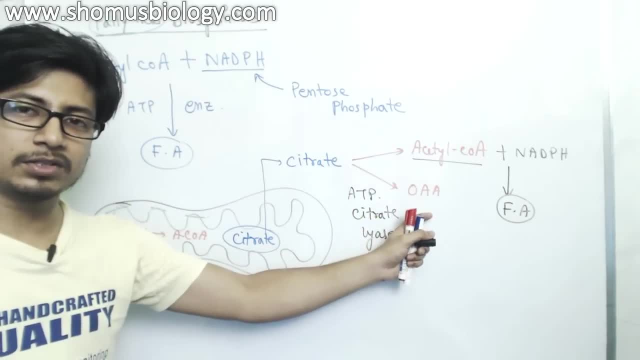 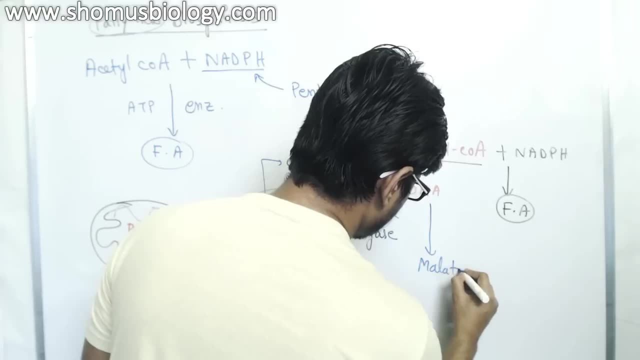 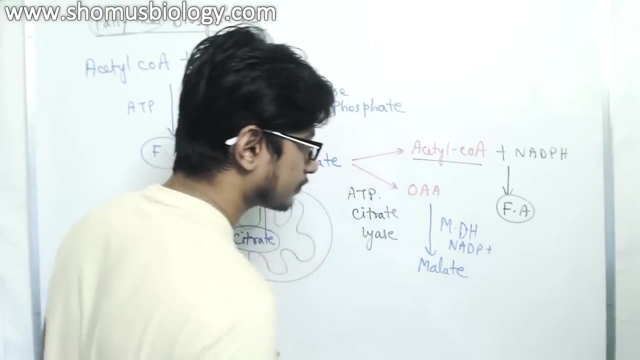 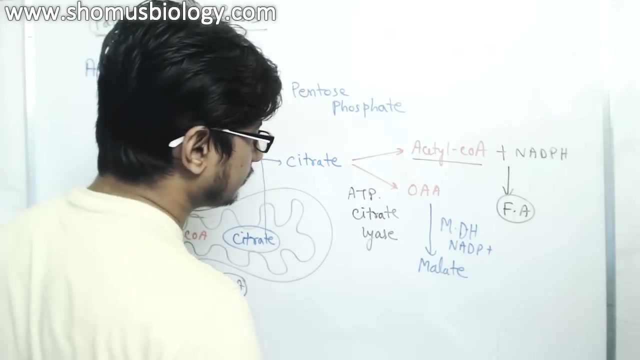 but what about oxaloacetate? we have oxaloacetate in the cytosol now. so oxaloacetate is further converted to malate with the help of malate dehydrogenase enzyme and in ATP help of malate dehydrogenase, oxidised acid can be converted to malate and then later. 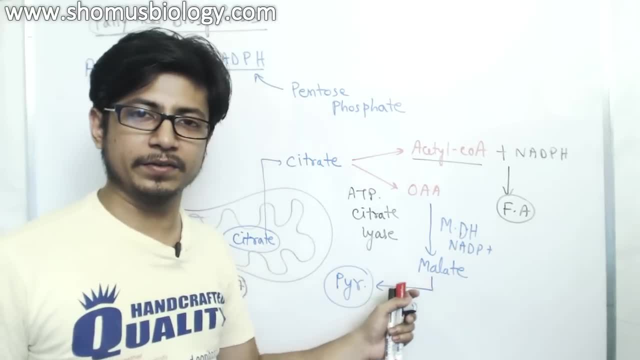 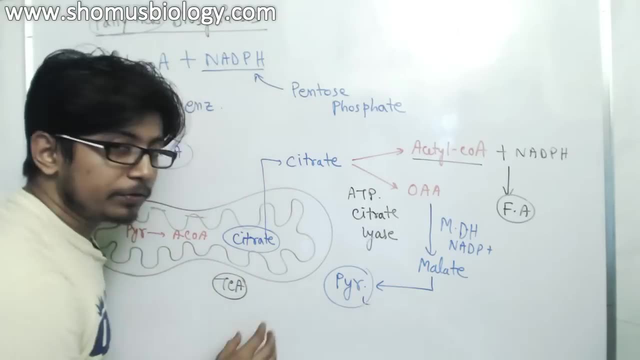 we can utilize malate to produce pirate. in the later stages. malate can be converted to private. it can be converted back to private and once the my�트, then this with the help of malate dehydrogenase enzyme and intoADP. 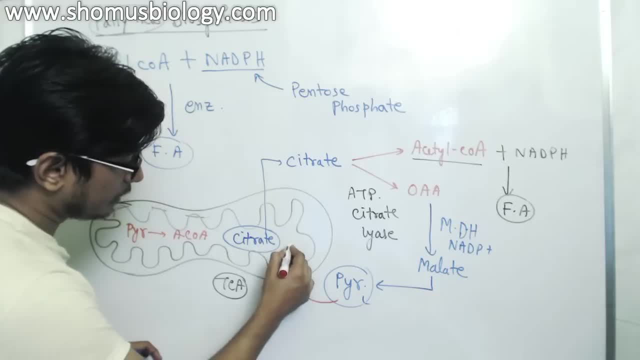 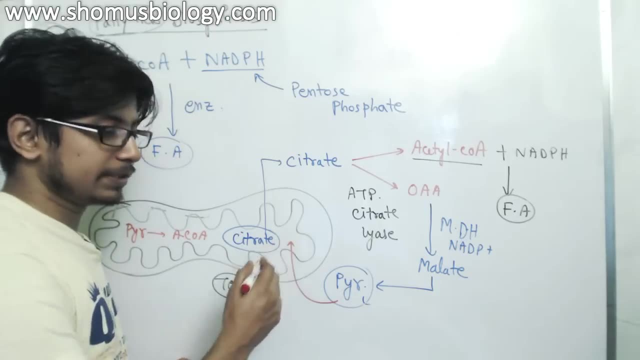 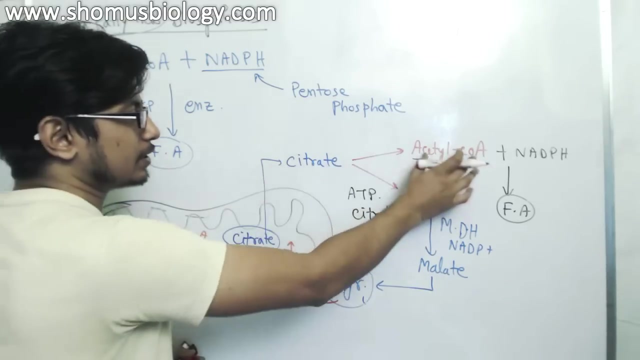 can be taken, and inside the mitochondria, because now the pyruvate can be converted into acetyl-CoA by pyruvate dehydrogenase complex in the matrix of mitochondria. So this is a cycle that goes on like that. It produces citrate, transport, the rest of the things, But ultimately we got our. 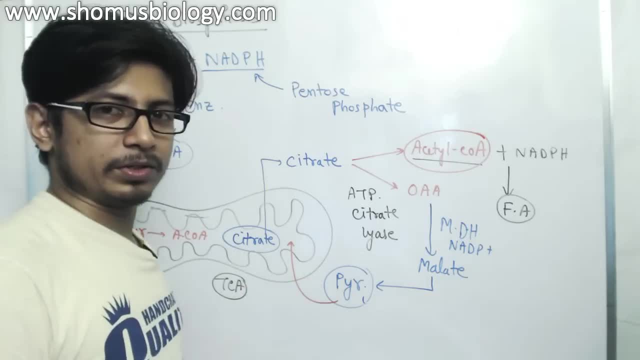 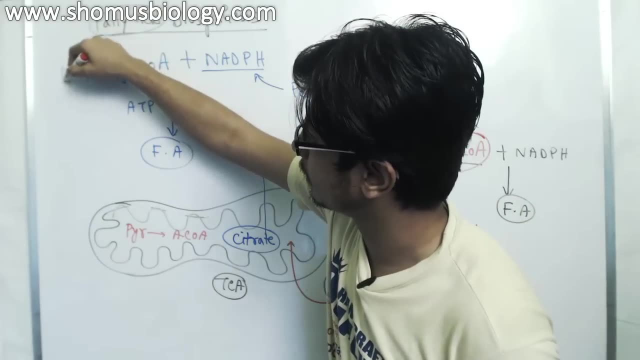 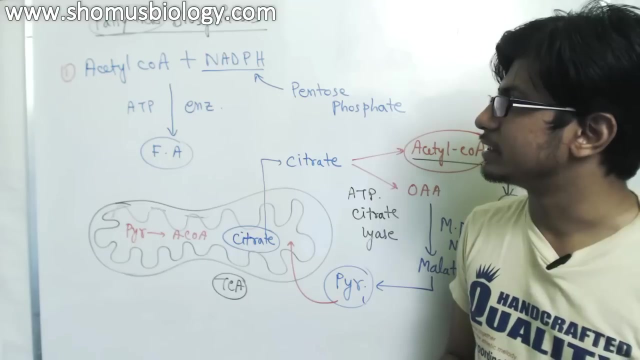 product that we need, And pyruvate is also an important intermediate that is produced at the end. So this is the process of the first problem to solve, that is a problem with acetyl-CoA. This is one thing that's very important, And the rest of the part about fatty acid biosynthesis is about. 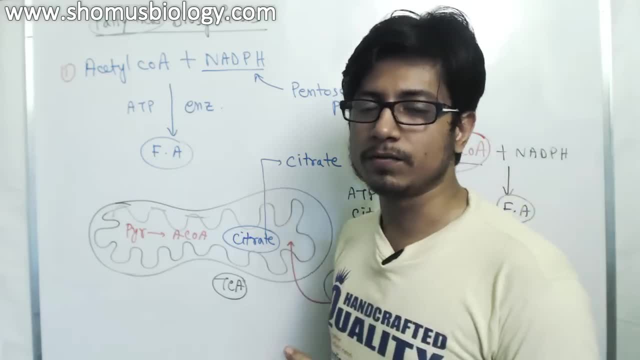 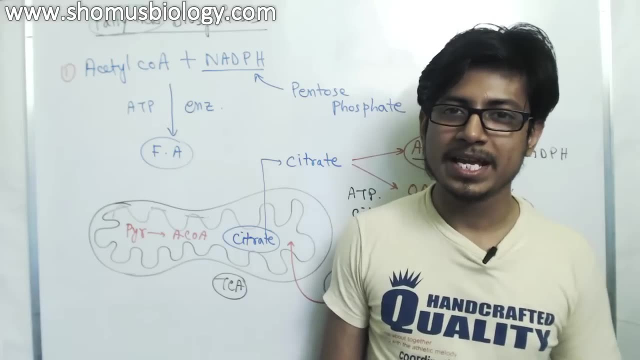 how exactly, for this biosynthesis pathway, is the length of the fatty acids? Because you know, fatty acids they are very long hydrocarbon chain that always form And the question about it. the second question that I want to ask is how exactly this such a long? 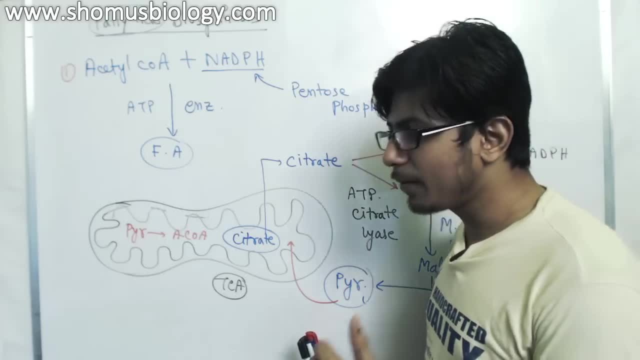 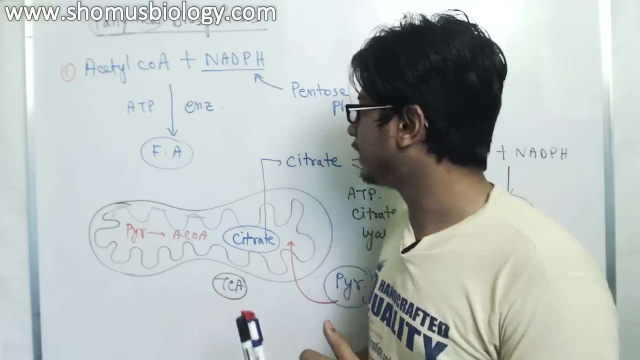 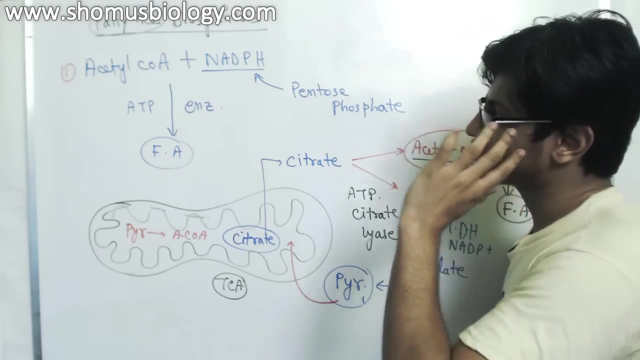 long hydrocarbon chains are formed And how exactly they make it more complicated, like triacylglycerols. The answer to that: if you think, the whole process takes place in the cytosol, So it carries some place in the cytosol, So it has acetyl-CoA and ADPH in there and start. 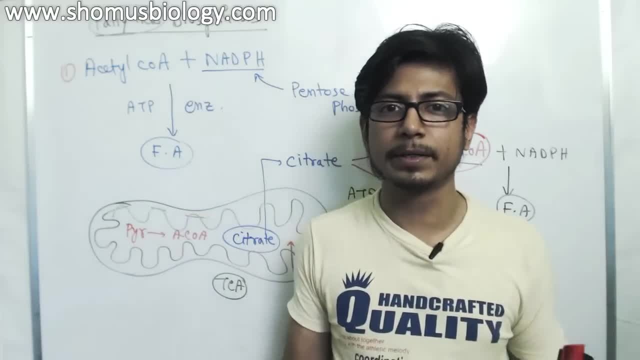 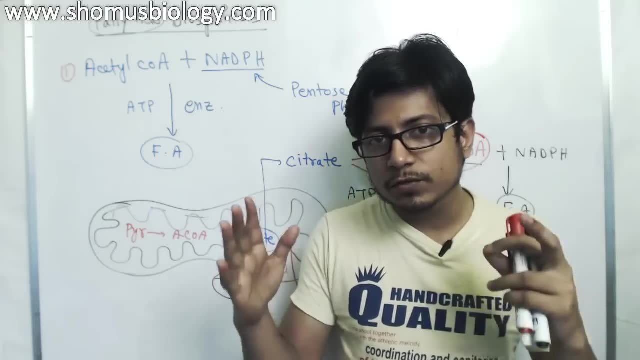 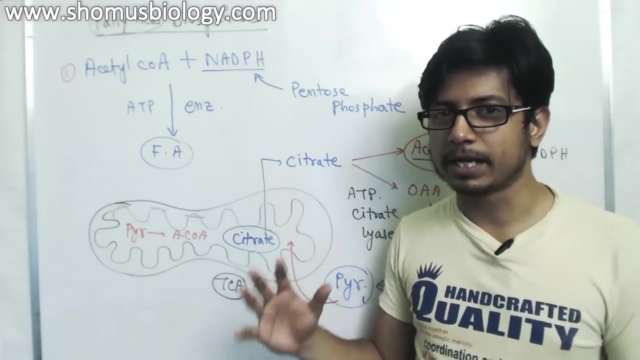 adding sequences with one another, But such a long hydrocarbon tail- cytosol- is where we have hydrophilic molecules around, So that is one big problem. So for a very short lipid chains- short to moderate length lipid chains- the process can take place in. 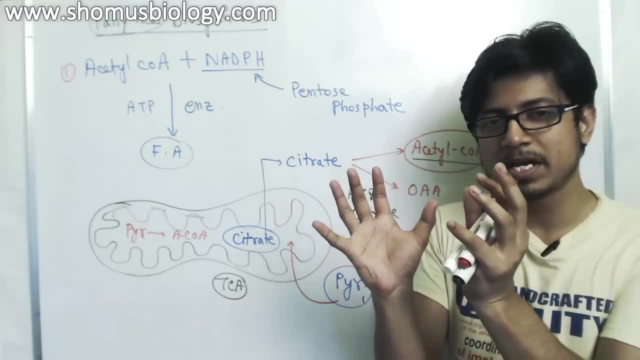 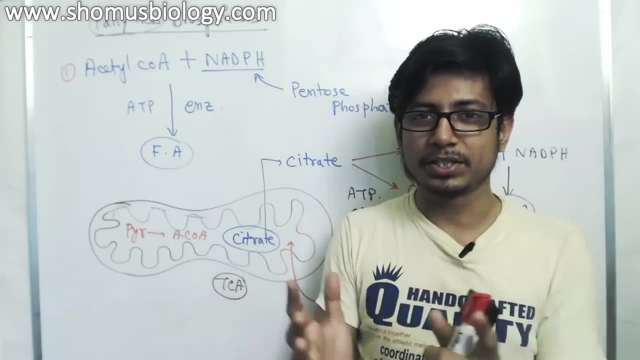 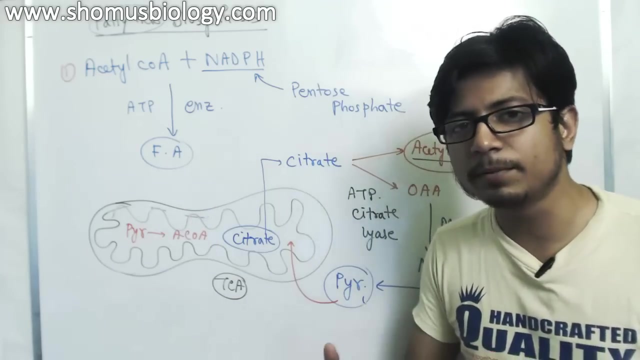 the cytosol with the help of other molecules engaging and involving with different hydrocarbon tail, which are hydrophobic in nature, to form mostly a separate mixture, separated out completely from the rest of the cytosolic component. It can stay there as spheres, But if the hydrocarbon 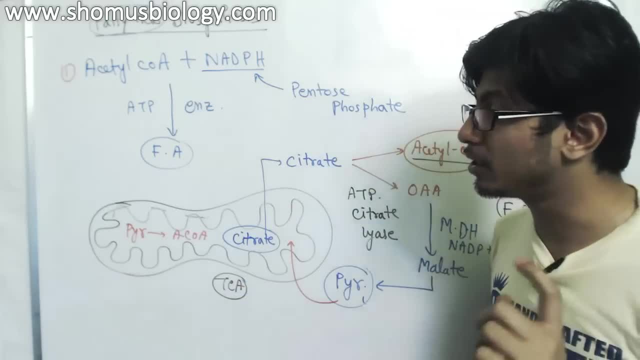 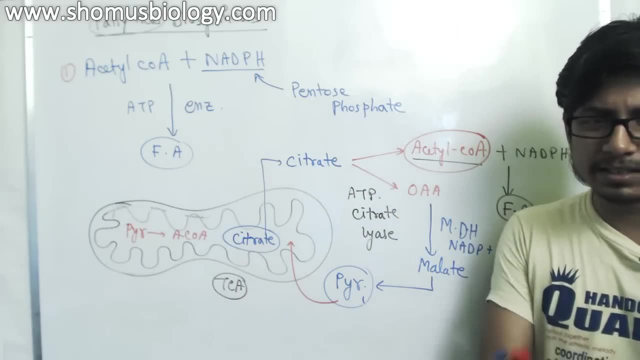 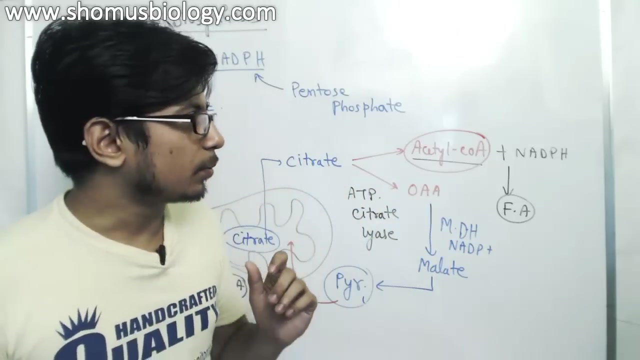 chain is really long. in those cases the process may not take place. So for a very short lipid chain it takes place in the cytosol. In that case it needs to use any other place, a separate compartment in the cell, to do the job. The third one, the third question that I told you that what about the? 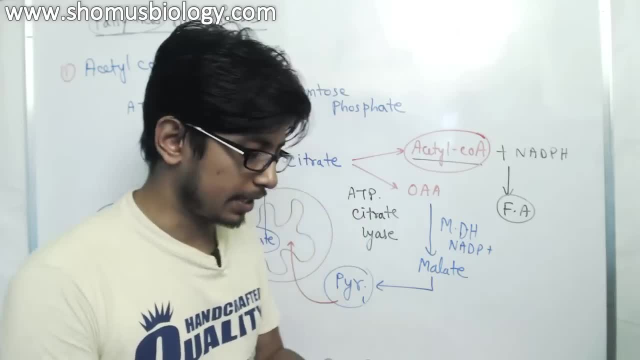 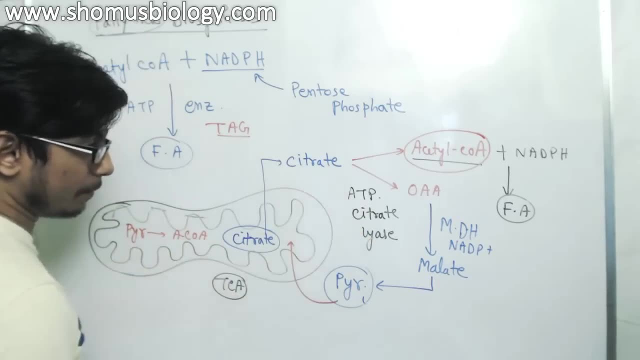 complex form of lipids, For example triacylglycerol. Triacylglycerol is not a unique fatty acid, where we have a glycerol backbone And along with the backbone we have three separate fatty acids linked. So for this type of structures, you know the glycerol that we are looking and talking about. 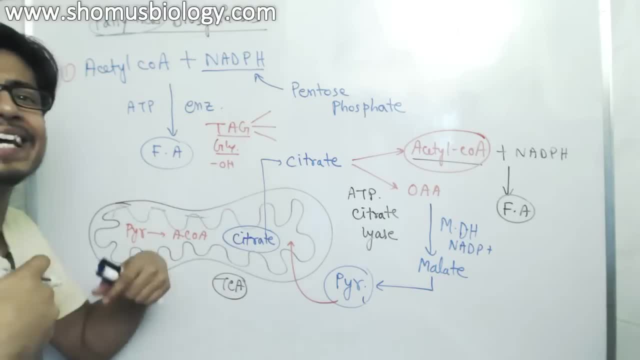 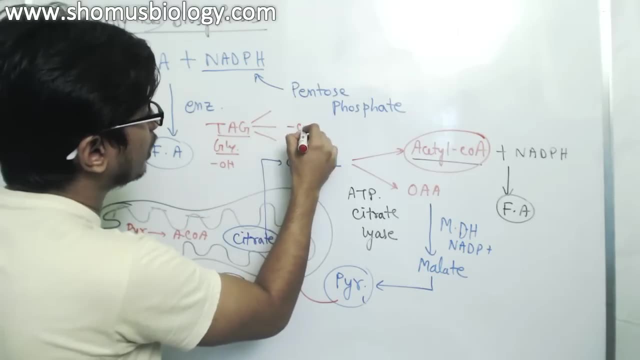 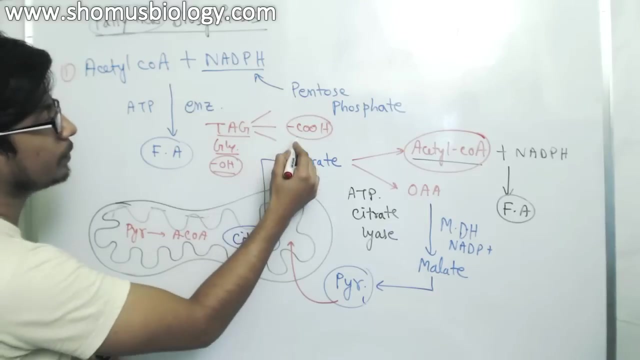 it is containing a hydroxyl group, hydroxyl bond. It's more like an ethanol type of thing, hydroxyl group, While fatty acids are organic acids, so they have carboxylic group, And it's nothing but the interaction between the hydroxyl group and the carboxyl group together to involve. 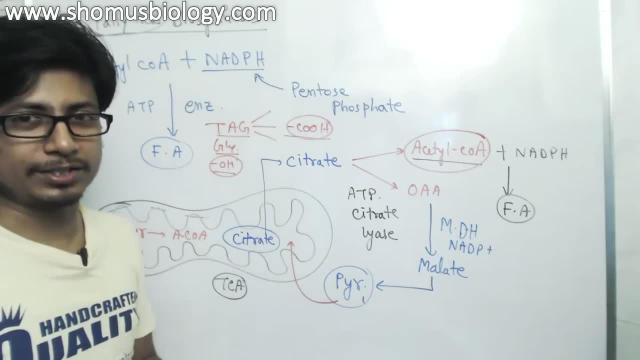 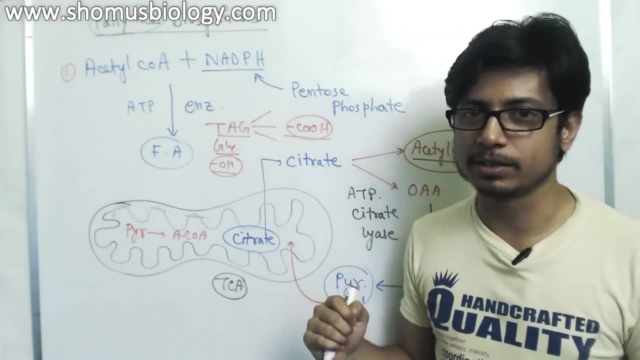 with themselves to form this triacylglycerol-like structures. So now, if you get an overview about the process, it's time to check the exact stages of fatty acid biosynthesis. And we not only see that, but also try to watch my video on beta-oxidation of fatty 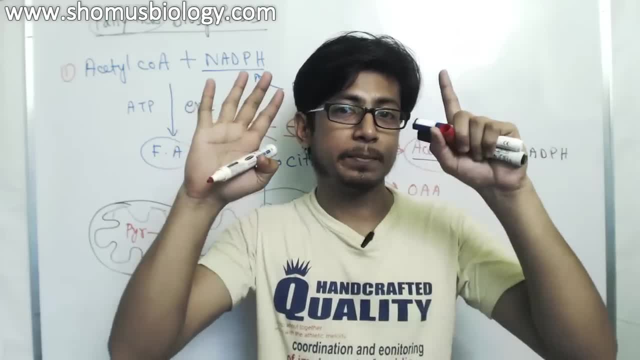 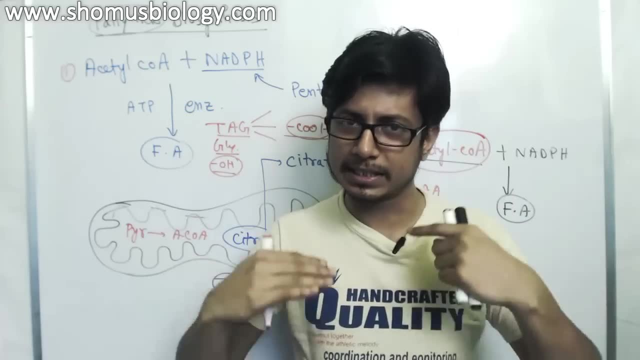 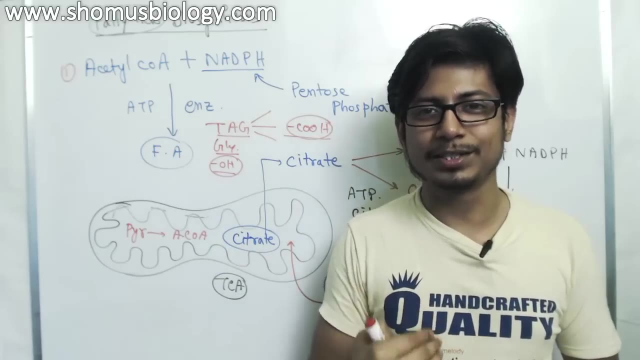 acid, And also the third video where I compare between the beta-oxidation and the biosynthesis of fatty acids, which you will see. most of the steps are very, very similar, with the same enzymes involved, but the little difference in the start and end steps and reaction stages. So watch this. 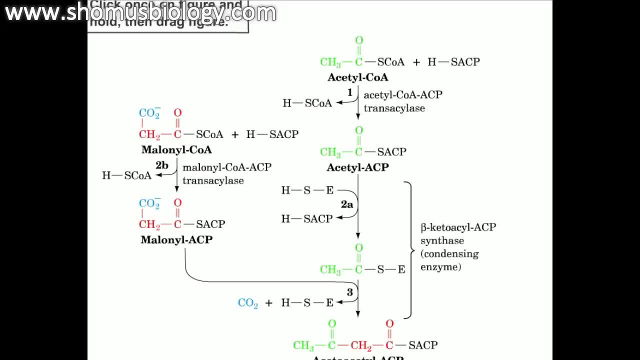 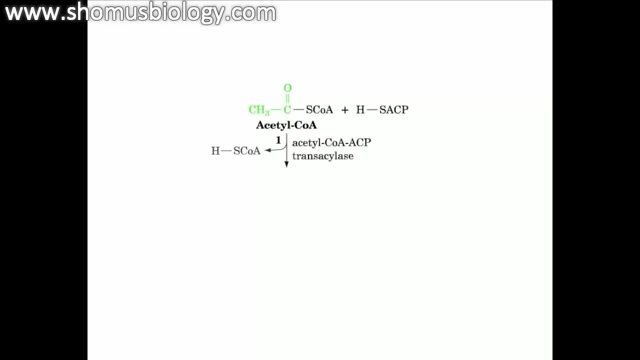 video And then check out the next. Let's look at the reaction sequence for the biosynthesis of the fatty acids. In the first step of the biosynthesis of fatty acids, the acyl carrier protein, or ACP, is very important. It plays an important role because this ACP is acetylated by acetyl CoA. It starts with acetyl. 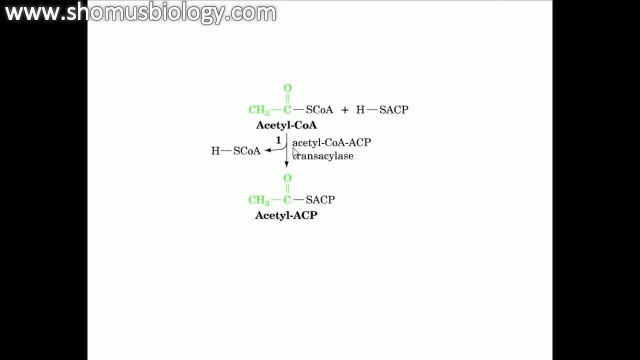 CoA. Once the acyl CoA or ACP is acetylated, the reaction produces acetyl CoA And then it starts with acetyl ACP And it is catalyzed by acetyl CoA. ACP transacylase enzyme. The second. 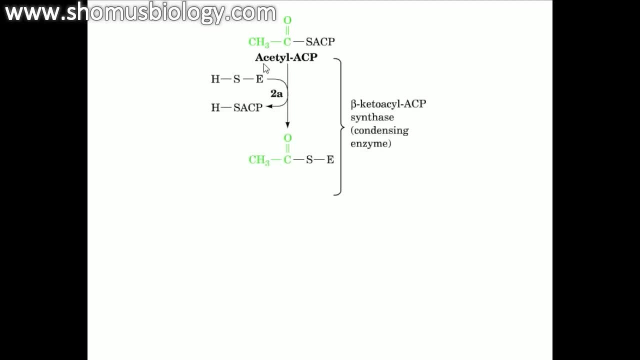 step is this: acetyl group of the acetyl ACP is transferred to the cis-sulphide group on the beta-ketoacyl ACP, And the enzyme involved with this process is beta-ketoacyl ACP synthase. Now 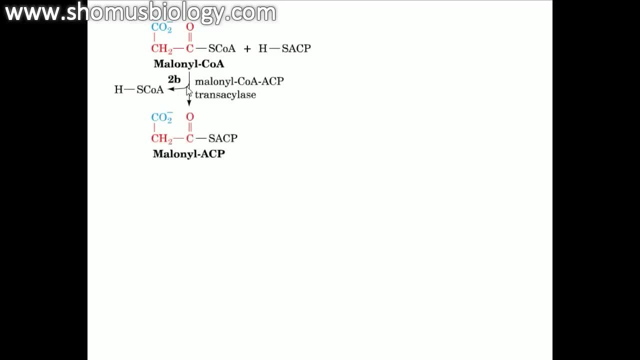 thirdly, the mannoline ACP. The mannoline ACP is produced from the mannoline CoA and ACP by the enzyme mannoline CoA- ACP transacylase. So it's simply, it's a transfer of the group ACP from one intermediate to the next intermediate throughout The acetylated beta-ketoacyl ACP synthase form a reaction. This from this reaction transfers its acetyl group to the mannoline ACP, which releases carbon dioxide. In the NADPH-dependent reaction, this acetoacetyl ACP is reduced to the d-beta-hydroxybutyryl. 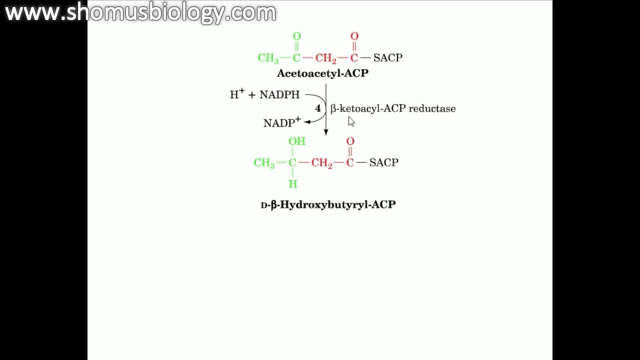 ACP by the beta-ketoacyl ACP reductase enzyme, And then this d-beta-hydroxybutyryl ACP is converted to the alpha-beta-transbutyryl or butanoyl ACP by the enzyme d-beta-hydroxybutyryl. ACP dehydratase. 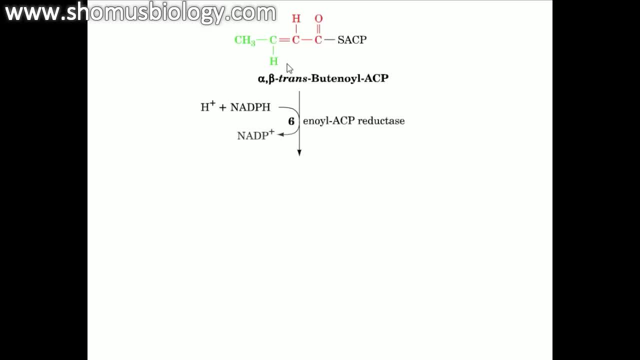